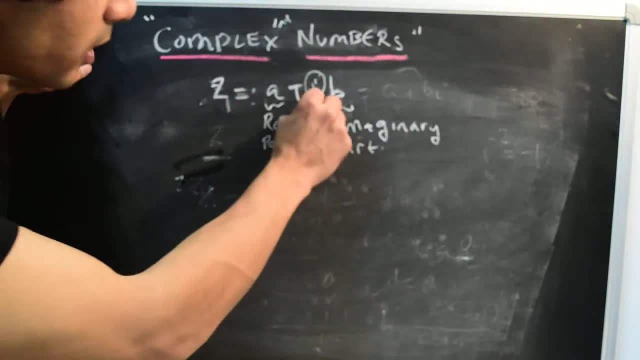 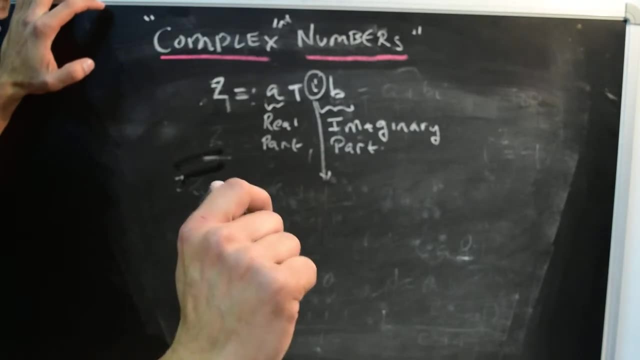 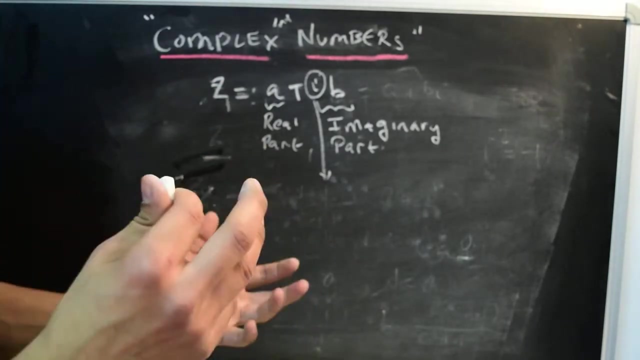 and an imaginary part. um, however, i here is to be taken more as a unit in the imaginary, uh, let's say- direction. now it's not at all obvious from this particular definition how to think about complex numbers as objects of this form somewhat more pictorially. that'll make it clearer how to, how to. 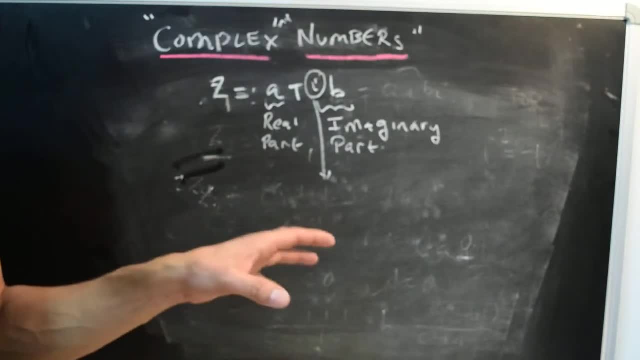 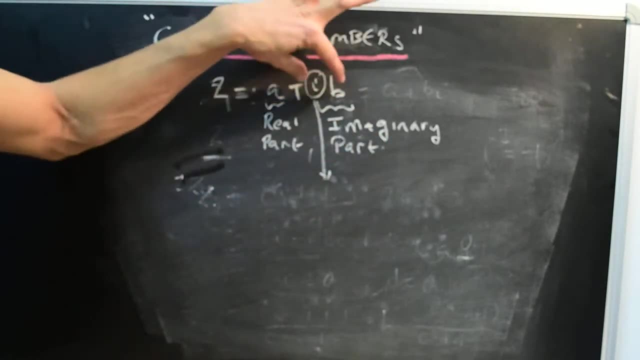 make a separation between the real and imaginary parts. but we'll get to that very soon. uh, we'll give it a give, a more geometric interpretation of what complex numbers are. but for now, what we'll do is: uh, we'll, we'll take this sort of symbol: uh, i with i, along with us, in some of the algebraic. 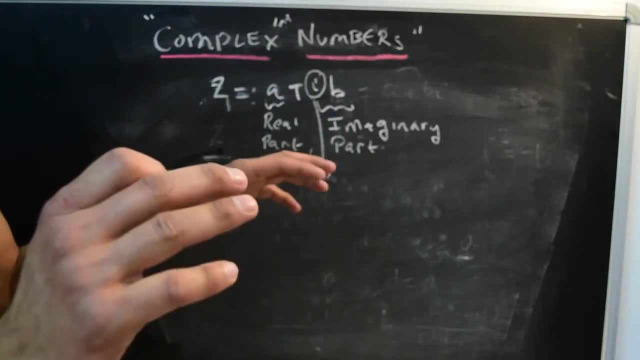 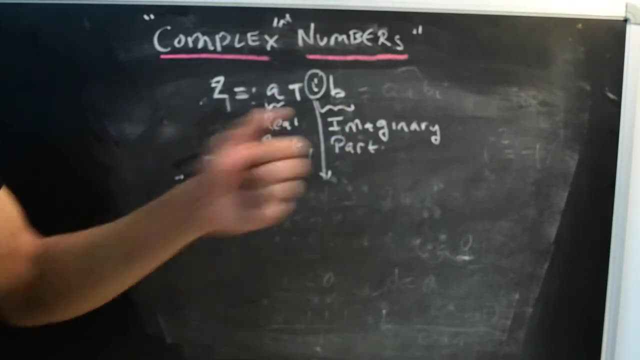 manipulations that we do, and what we'll say is that i denotes, uh, some kind of a unit. uh, this identify a real part and an imaginary part, but the imaginary part itself is actually the real number b that sort of gets attached with the symbol i. So, somewhat more precisely, 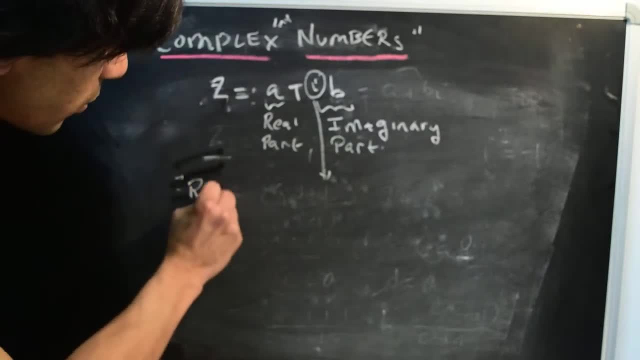 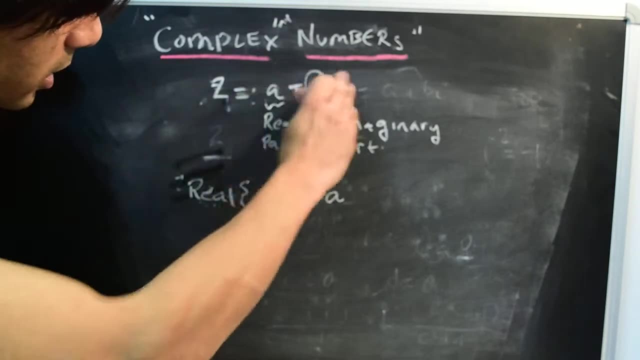 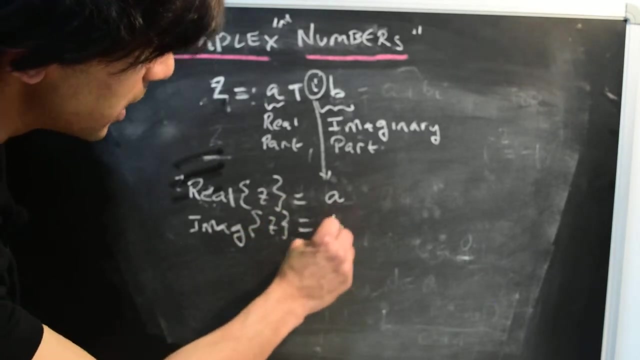 if you are asked like what is the real part of z, we will say that the real part of z is simply the real number a, which doesn't carry with it the symbol i in this case, and the imaginary part of z is the real number b. So notice that a and b are both real, So a. 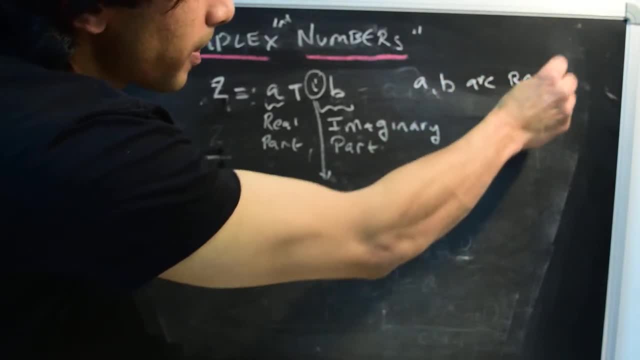 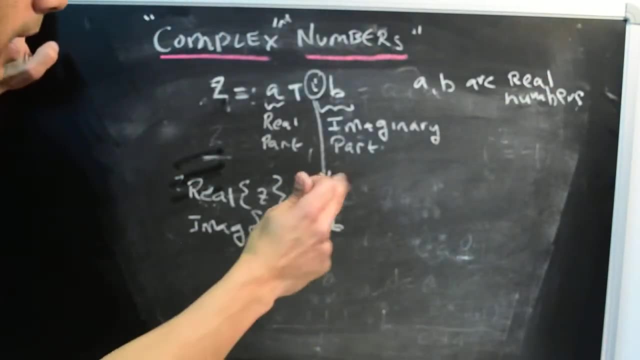 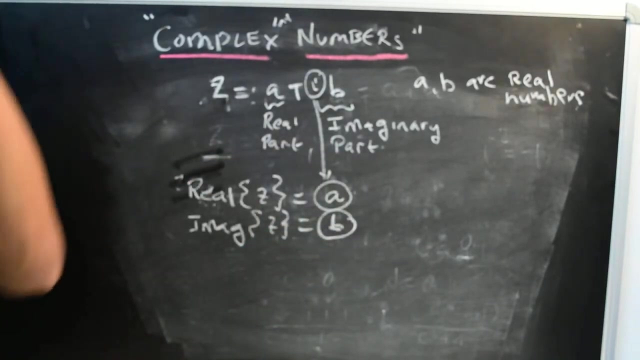 and b are real numbers, So i is simply a symbol or a unit that helps identify the imaginary part in this complex object, and the imaginary part itself is actually the real number b, and the real part is the real number a. Now, one of the things that we will do here is that we will sort of now try and introduce 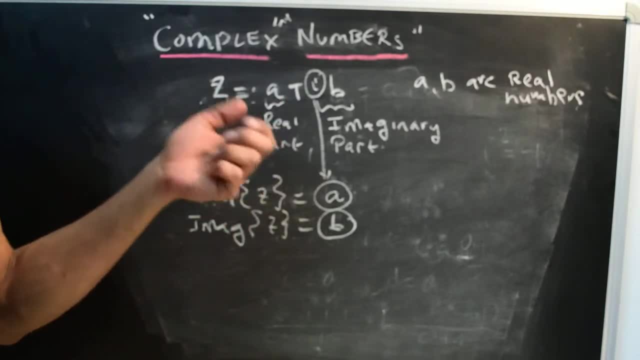 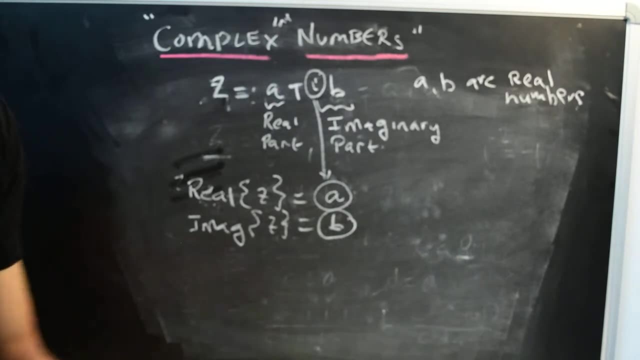 or make some definitions of how to carry out algebra with these complex numbers, In the sense that we will now define addition, subtraction, multiplication and division of complex numbers. There are certain sort of steps in that definition that will help us identify the imaginary part. 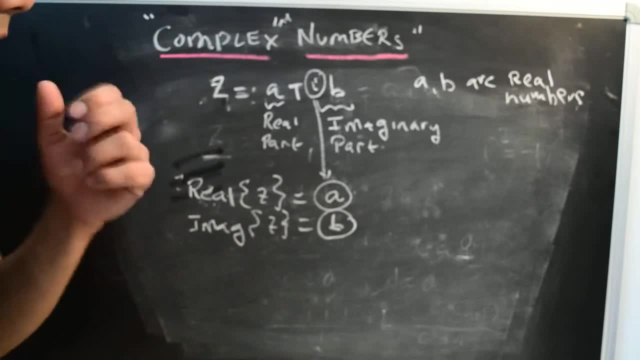 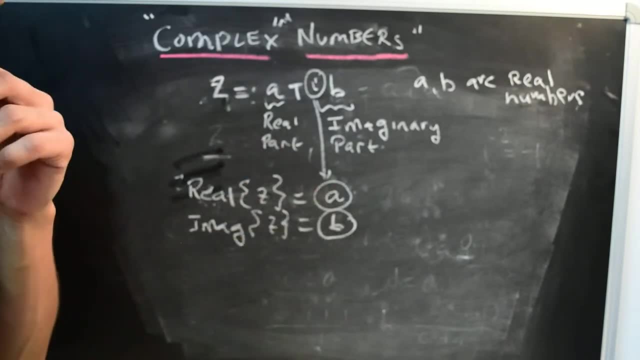 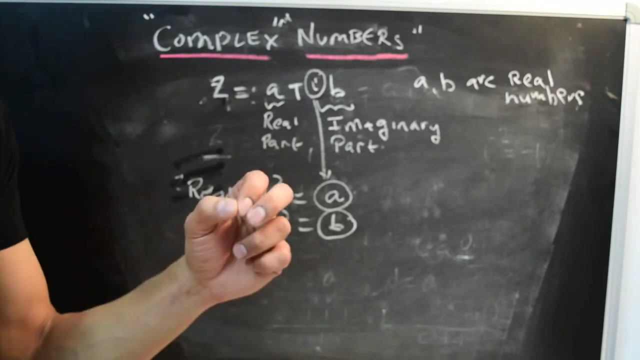 that will assume, that will make assumptions about how we work with the symbol i, And these are assumptions in the sense that we won't be able to justify them from first principles. but what we will claim is that if we accept these definitions for addition, subtraction, 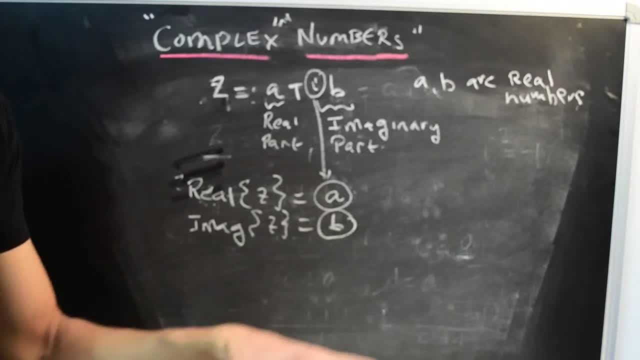 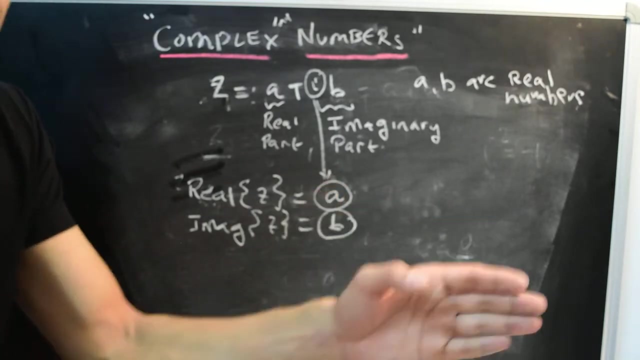 multiplication and division of complex numbers. then complex numbers or these complex objects follow all the rules of algebra, So we will be able to identify the imaginary part of the rules that we established or that we chose to identify any kind of number with. So, given an object, if that object satisfies the set of rules we listed out in the previous videos. 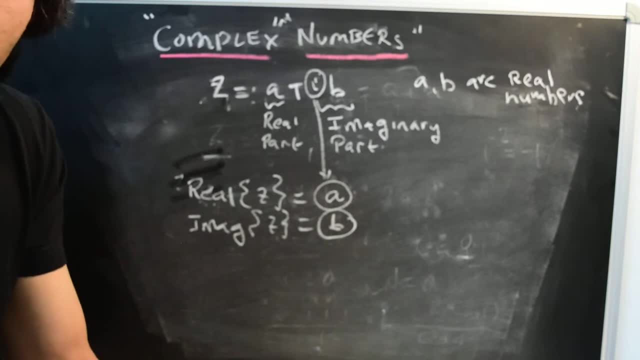 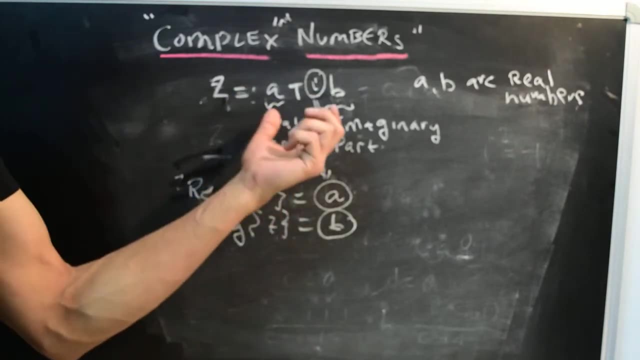 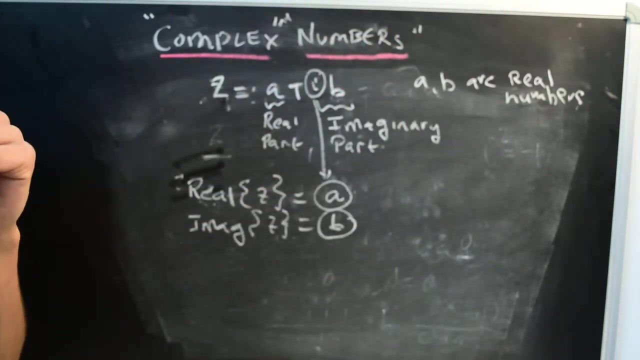 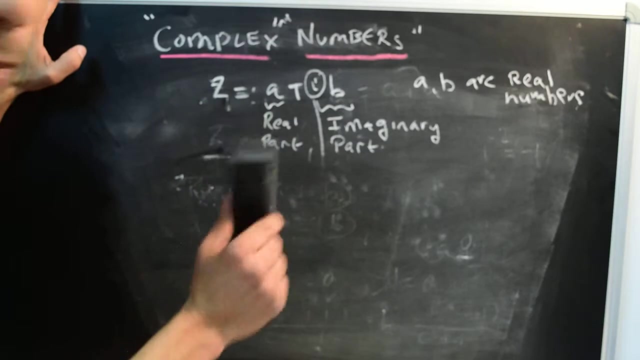 we will choose to call such objects as numbers. So with the definitions that we will make, it turns out that these complex objects will satisfy all those rules and therefore we are calling such a complex object as a complex number. So let's just work out how that works and it will make it clear where some of the assumptions 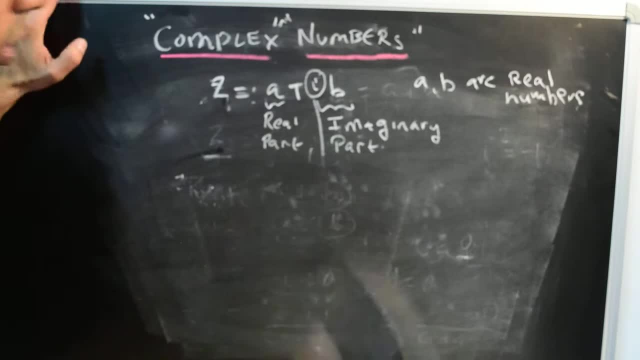 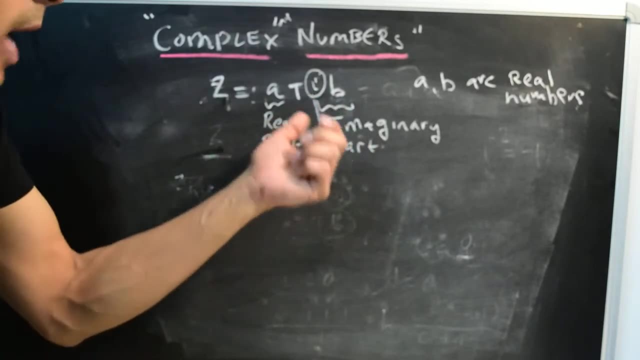 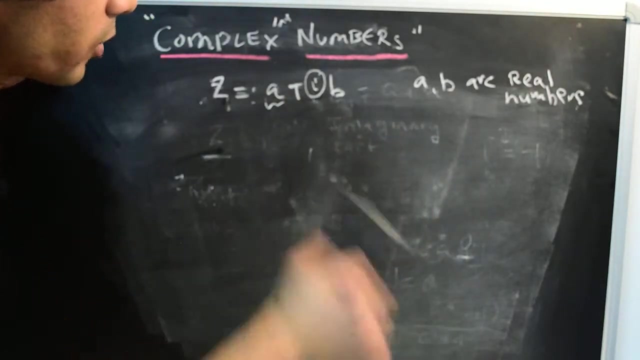 that we are making enter the picture. So just to recap here, the real part is the real number a and the imaginary part is the real number b and an. i sort of helps us identify the imaginary part in this complex object. So now let's see how do we define the addition of complex? 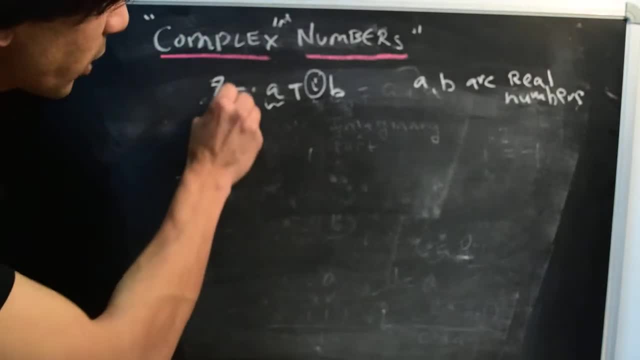 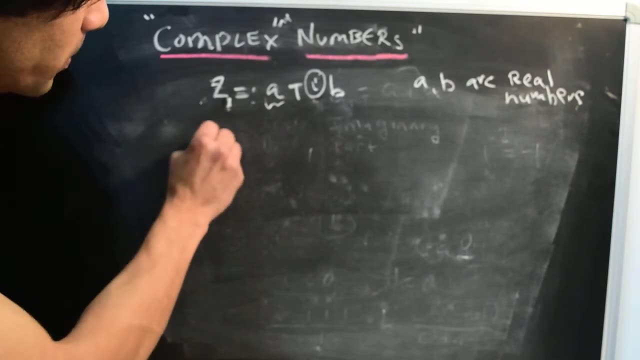 numbers. So let's start with addition and subtraction of complex numbers. So let's say we are given one complex number, z1, which is again of the form a plus ib, and another complex number, z2, which is of the form c plus id. then the way we define the addition of complex 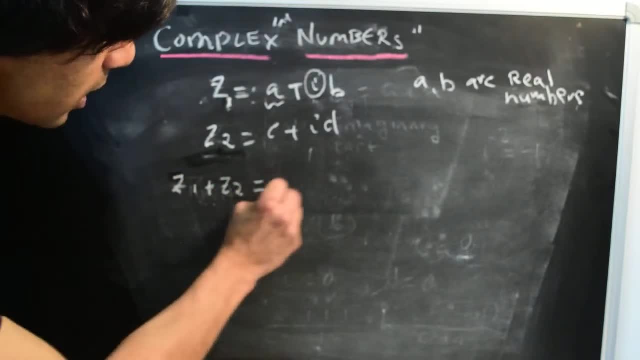 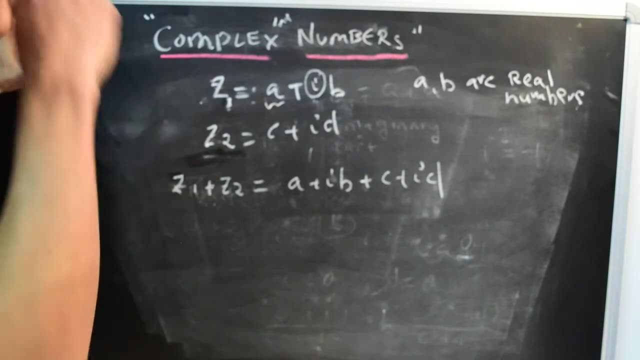 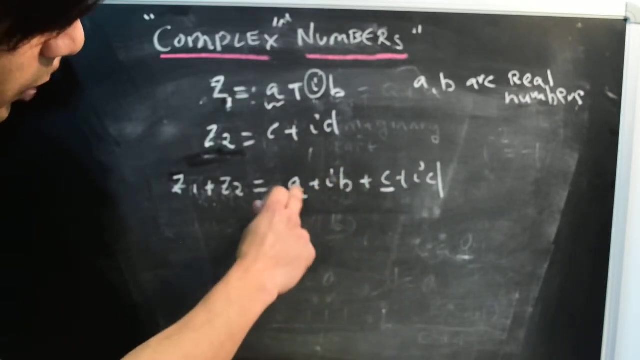 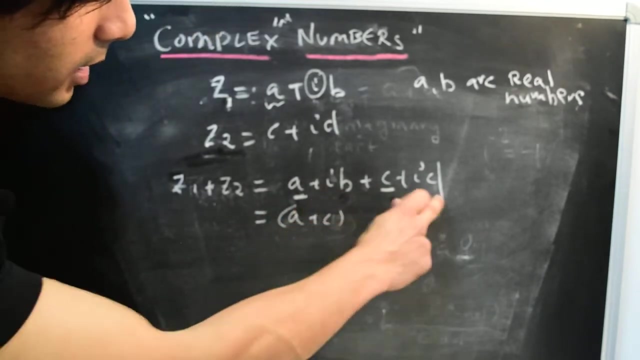 numbers is that the sum z1 plus z2 is a plus ib, plus c plus id, and then what we do is we can sum. we again have something that carries. we have an a and a c, which are both real numbers, so we can simply add them, so we have a plus c, and then we will identify the symbol i in. 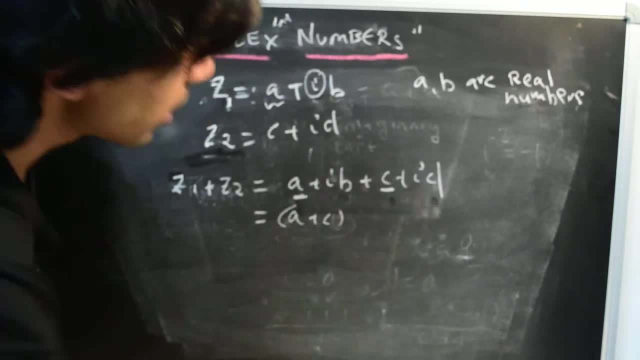 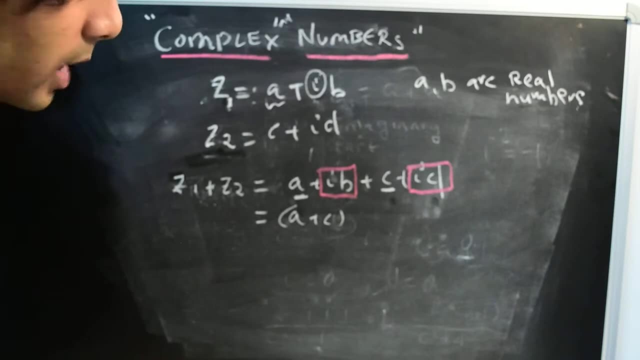 this expression. so we have two expressions that carry the symbol i, ib and id, and what we will do is we will combine these two together. so we will write this as i times b plus d, And notice what happens if we make this definition for addition of complex numbers. what happens: 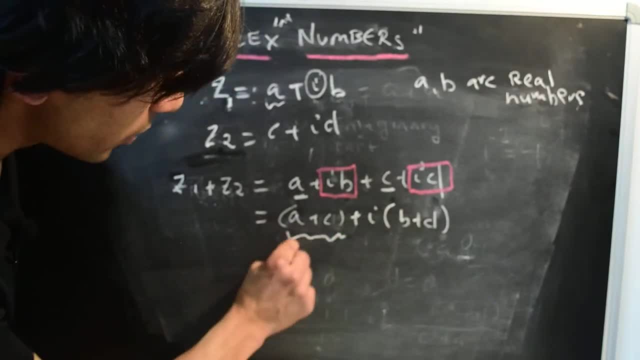 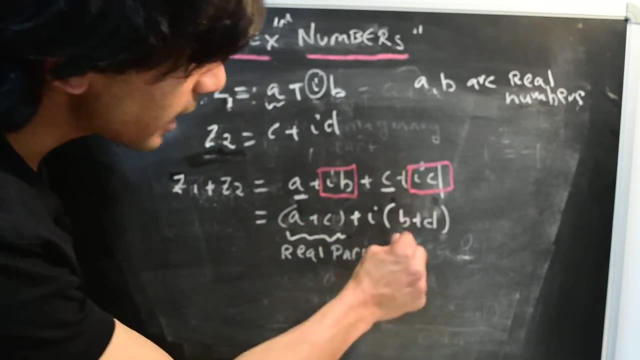 is that we again have an object that looks like it has a real part, which is a plus z, so that's a real part, which is the sum of two real numbers. so a plus c is also a real number. and then it has an imaginary part, which is b plus d, and b and d are both real numbers. 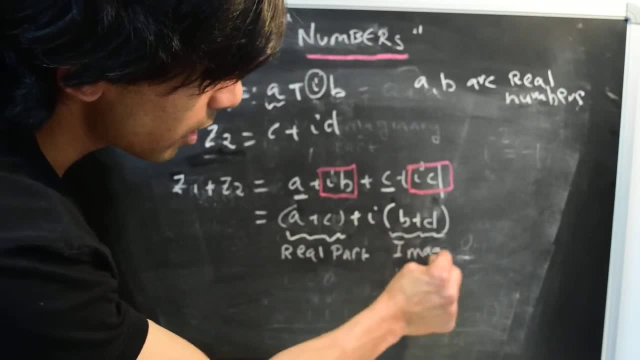 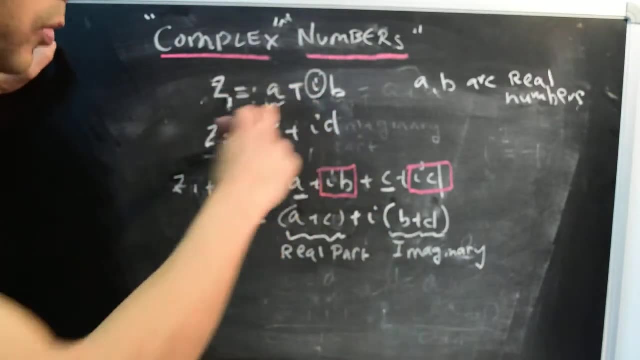 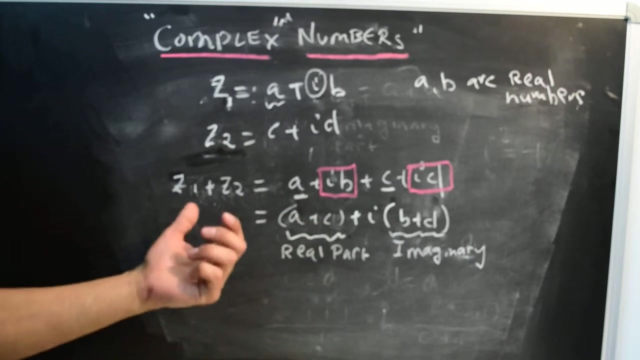 so this is also a real number, so this is the imaginary part, And therefore this composite object also looks like what we define as a complex number, which is it has a real part plus i times an imaginary part. and therefore what happens is if we make this definition, then z1 plus z2 gives us another complex number, and because of the fact that, 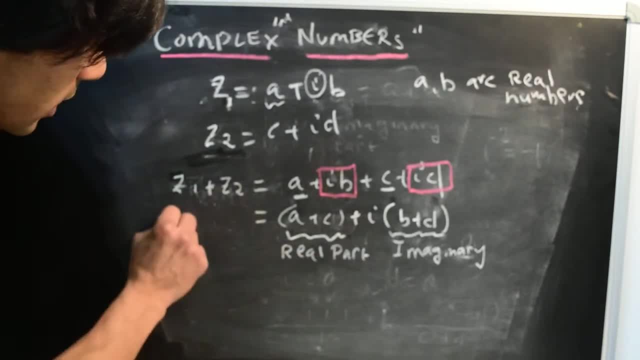 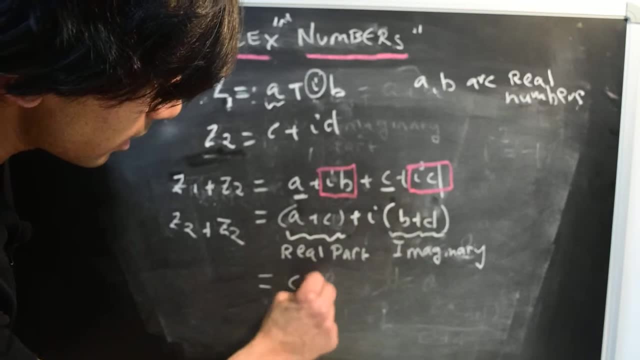 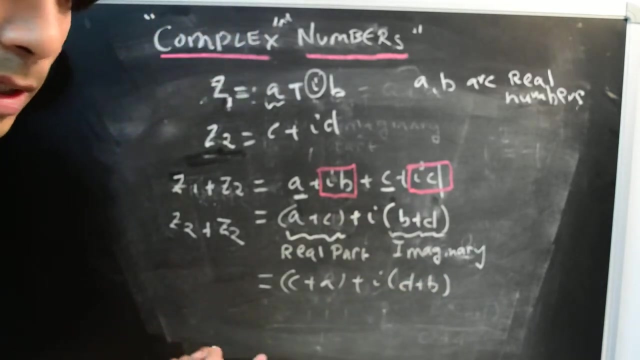 real numbers commute, we find that z1 plus z2 is also equal to z2 plus z1, because z2 plus z1 will give us c plus a plus a. i times d plus b. right, so sorry, let's write this as z1 plus z2 and this is z2 plus z1. 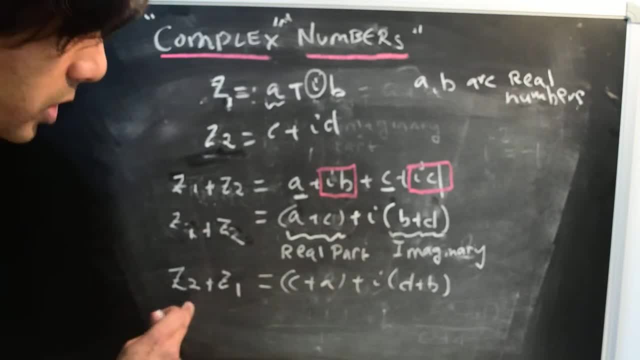 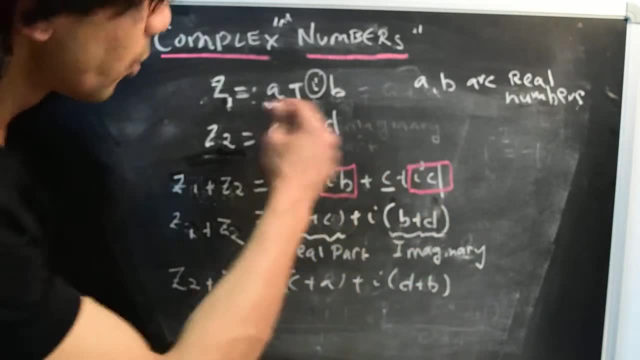 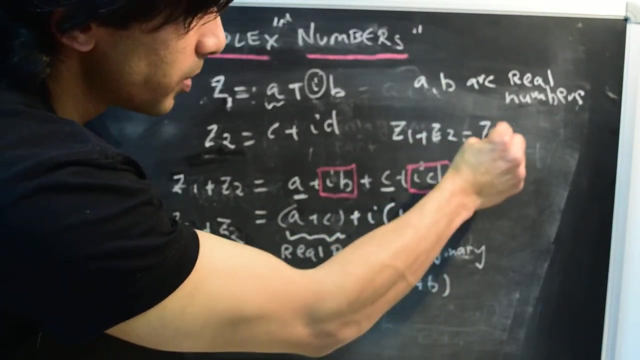 and because real numbers commute, we find that z1 plus z2 is actually equal to z2 plus z1, because a plus c is equal to c plus a, and b plus d equals d plus b, and so, with this definition of complex numbers, we'll find that z1 plus z2 is actually equal to z2 plus z1. 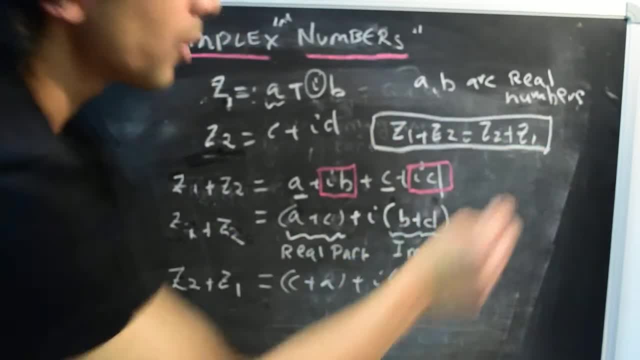 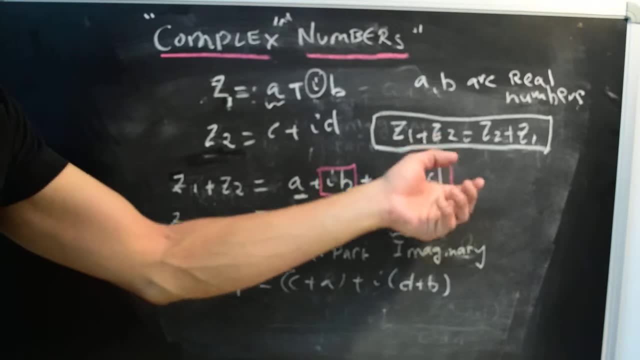 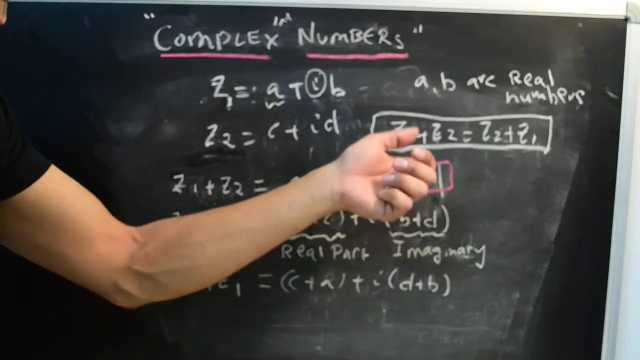 plus b, which is one of the rules with which we, if an object satisfies- this was one of the rules that the object needs to satisfy for it to be called a number, and this rule is again called is called that addition is commutative. so again we'll say that, given 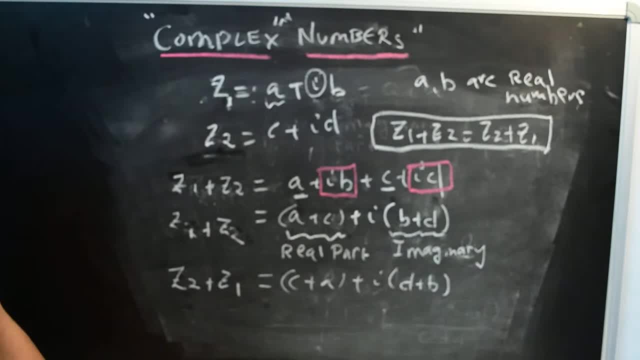 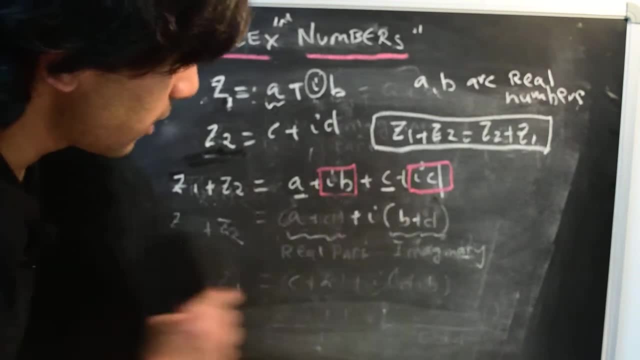 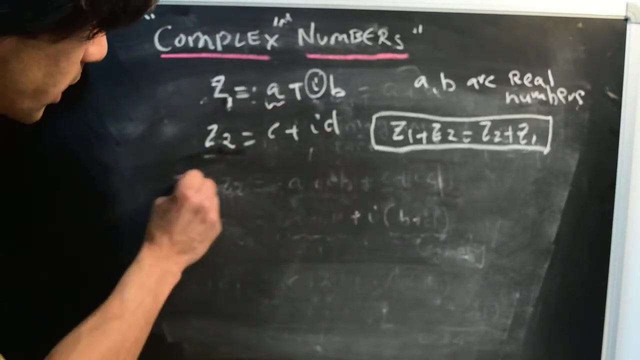 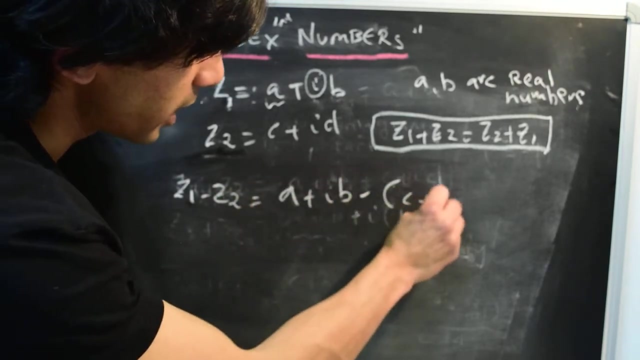 this definition of complex numbers. their addition is commutative. alright. now, in the same way, we can carry out subtraction of complex numbers, and what we'll do is so we need to define z1 minus z2. so if this is z1, this is z2, then z1 minus z2 is a plus ib, minus c plus id, and again we can combine the. 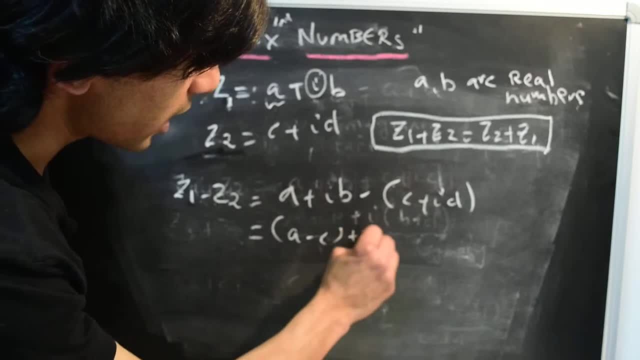 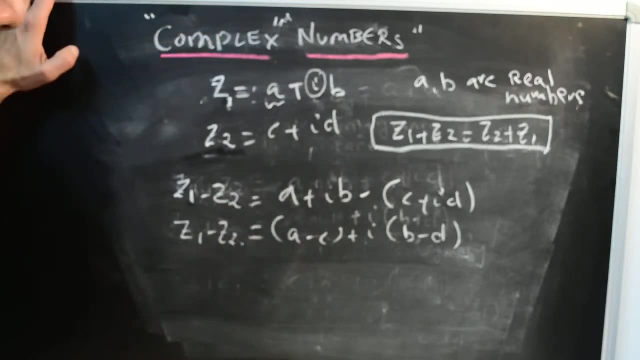 real and imaginary parts. so this will give us a minus c plus i times b minus d, and that's z1 minus z2.. And again this composite object looks like another complex object because it has a real part plus i times an imaginary part. so this is another complex number. 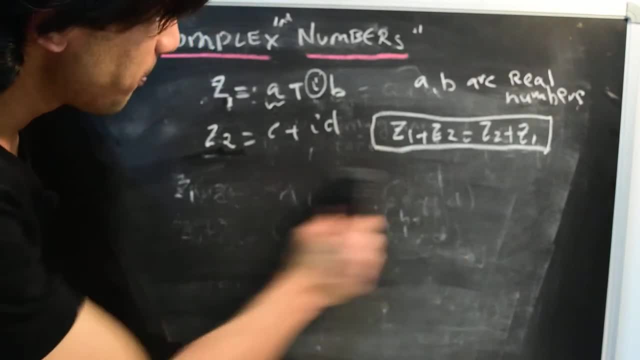 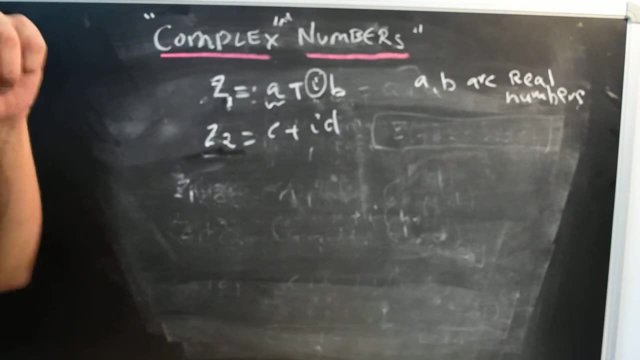 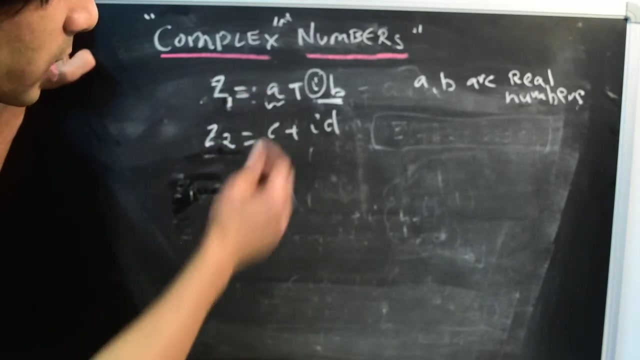 Okay, Great. So the next step is to define multiplication of complex numbers. actually, before doing that, there's one important point which is well: given a complex number, let's say z1, which is a plus ib, or z2, c plus id. Okay, 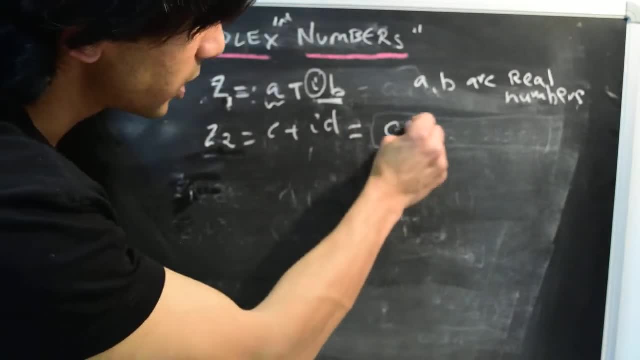 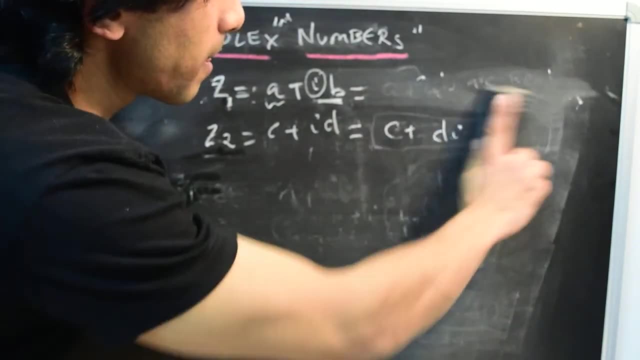 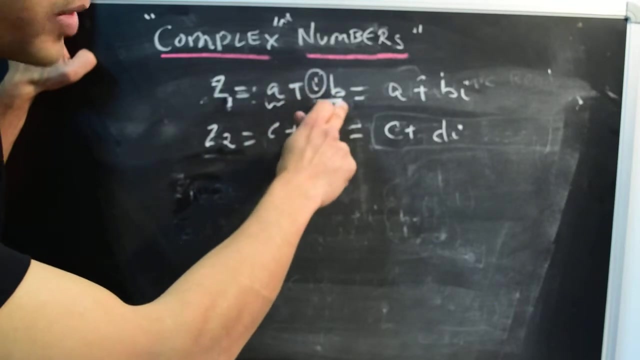 equal to. we claim or we say that this is equal to C plus D times I and this is equal to A plus B times I. So it doesn't matter on which side of the real number B we write A. Now this is not at all obvious. What we are claiming here is that the symbol I, which 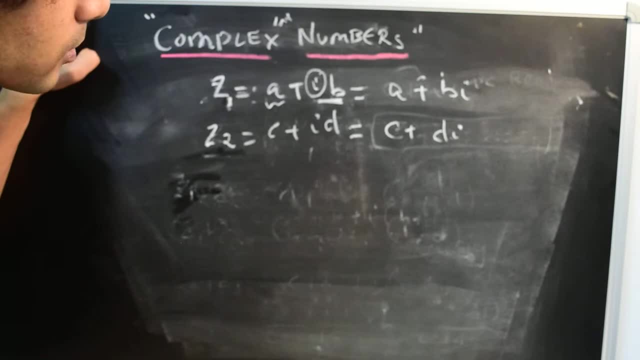 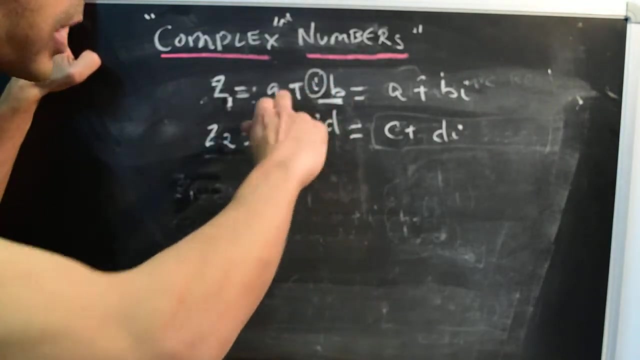 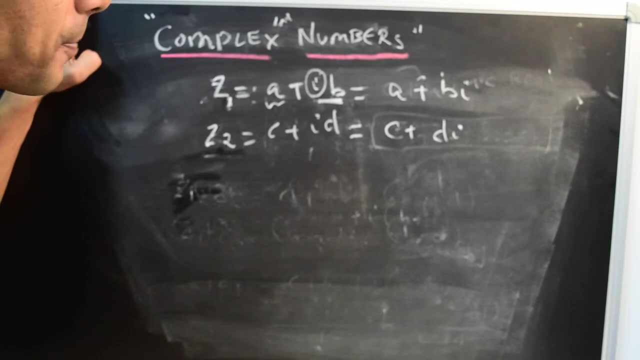 is the unit imaginary number commutes with any real number it appears with. So this we will take to be sort of a definition that, given a symbol, I we can sort of move it around the real numbers that it's coming along with. So with this sort of definition, let's define. 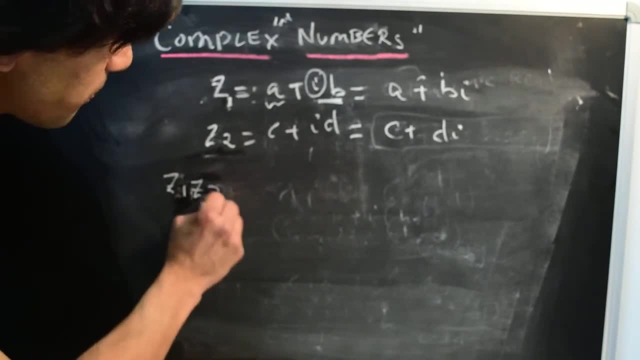 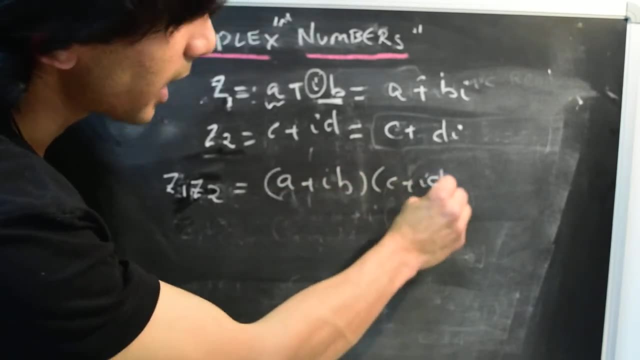 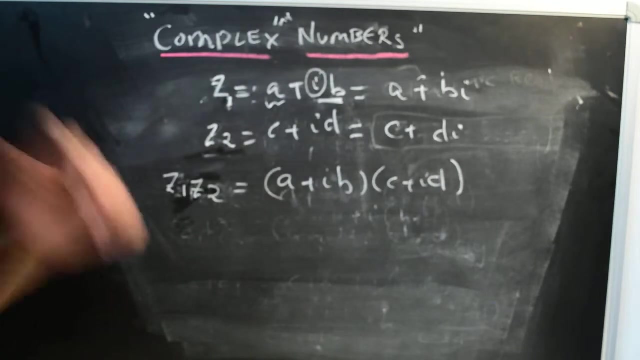 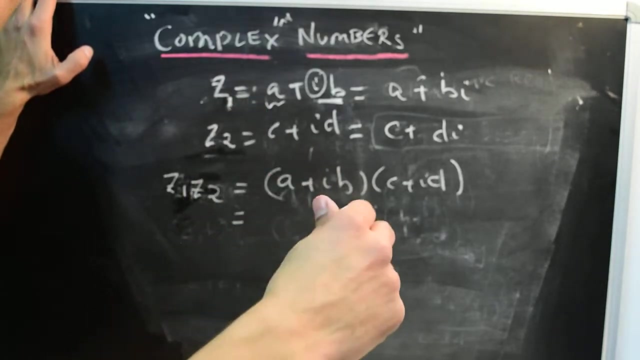 a multiplication, complex, Complex numbers: Z1 times Z2 is A plus IB times C plus ID, and actually this rule is not sort of this rule, or rather multiplication is sort of a generalization of this definition. So now what we'll do is we'll say that, okay, we know that real numbers distributes multiplication. 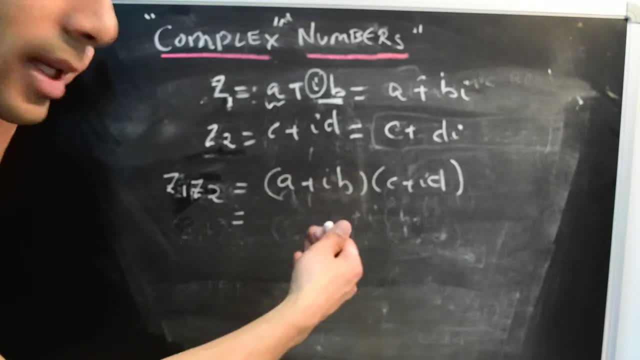 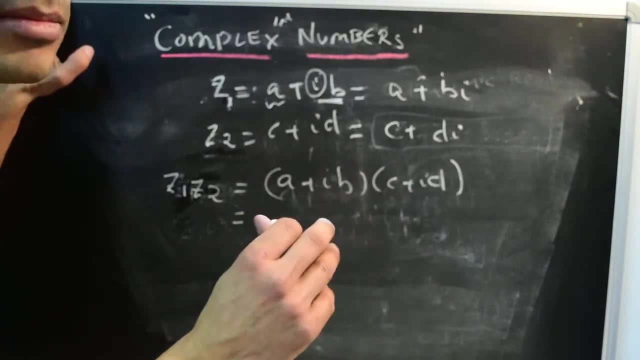 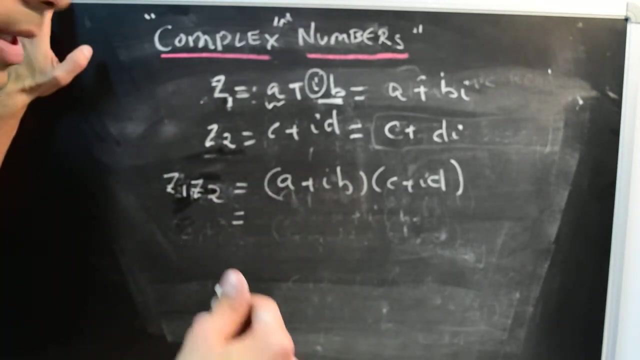 of real numbers distributes over addition. and in making this definition of multiplication of complex numbers, We'll say that I sort of carries along as a symbol for a unit imaginary number, but it doesn't change or we are still allowed to use the property that if you are multiplying, 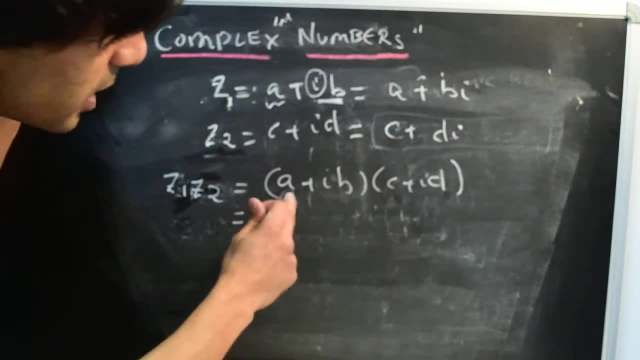 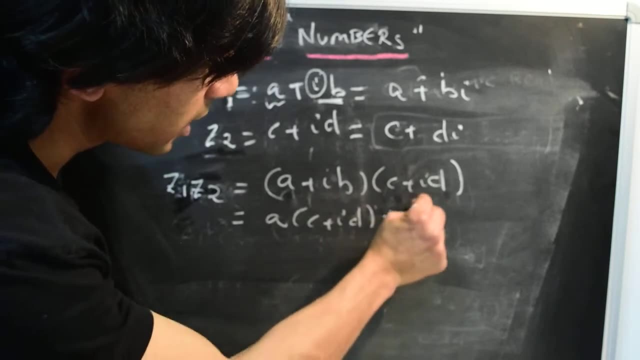 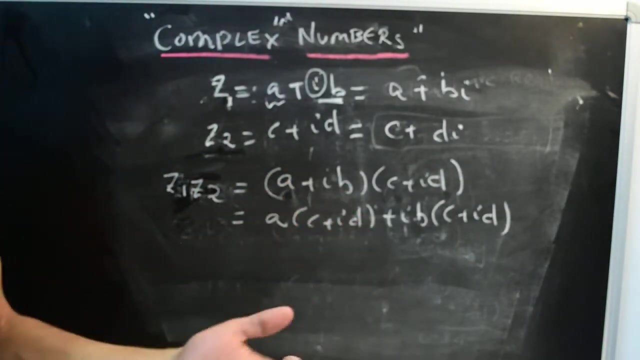 A with C plus ID. So, for instance, in this case, what we'll claim is that we can write this product as A times C plus ID plus IB, times C plus ID. So we are working with this symbol I, as if we are just, as if you are working, as if you are working with any other. 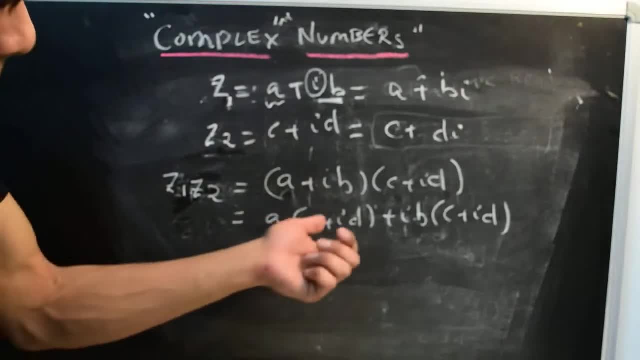 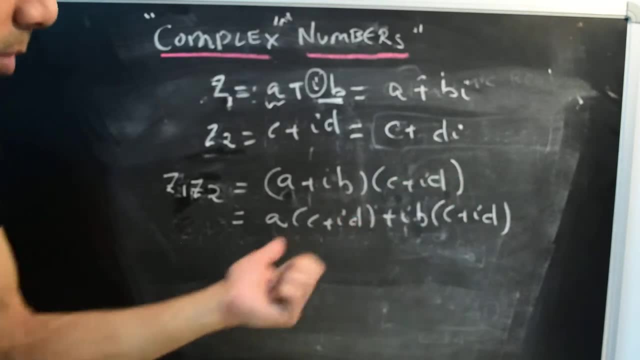 number like the real number that we are familiar with. So we are still claiming that, okay, A and this sort of composite sum, A plus IB, and its product with C plus ID, can be written in the form: A times C plus ID plus IB, times C plus ID. So this is part of the definition. 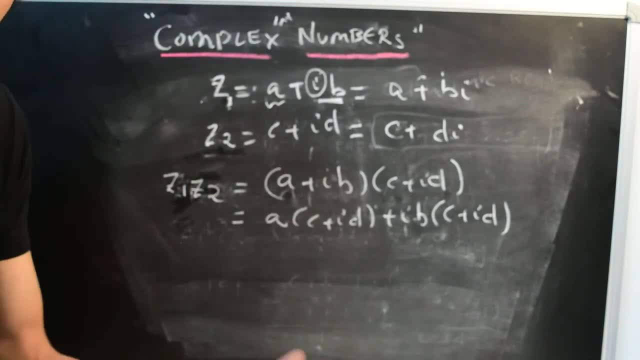 that we are making for multiplication of complex numbers. It's not at all a first principle derivation of why we are allowed to, for instance, commute I with B and why we are allowed to make, why we are justified in picking out this IB and writing it as or multiplying this. 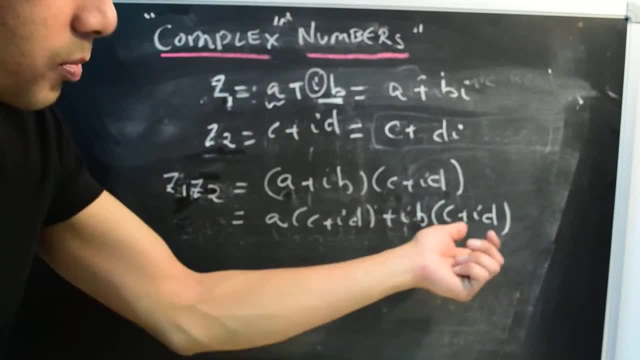 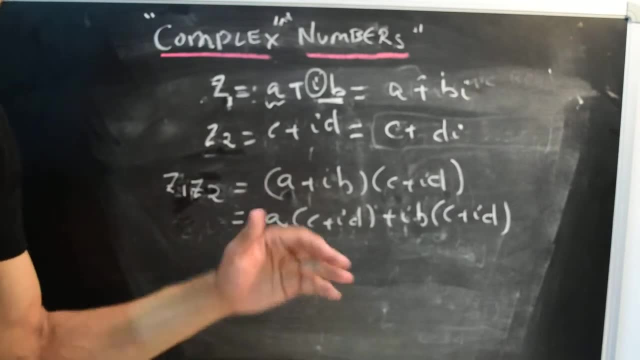 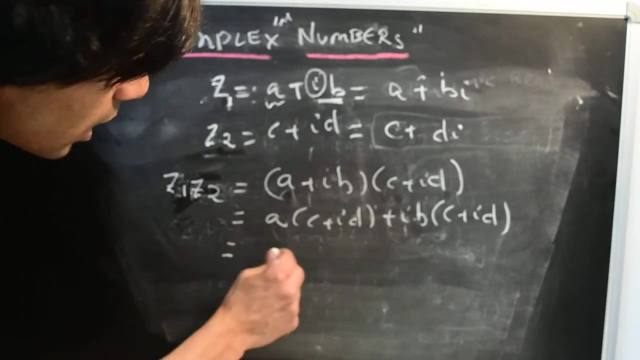 with C plus ID and then distributing this product over addition, as we'll do in the next step. So these are not first principle derivations. this is just a definition of multiplication and we'll give it a more geometric meaning in subsequent videos. So, given this definition, 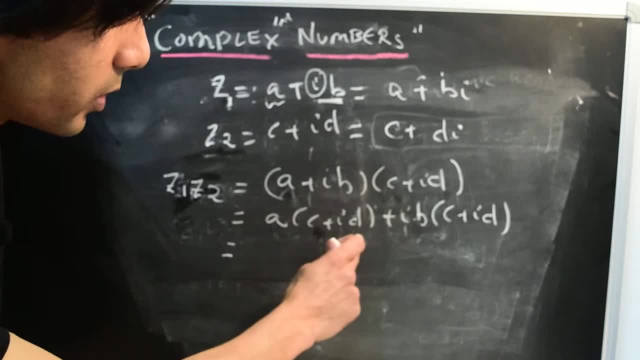 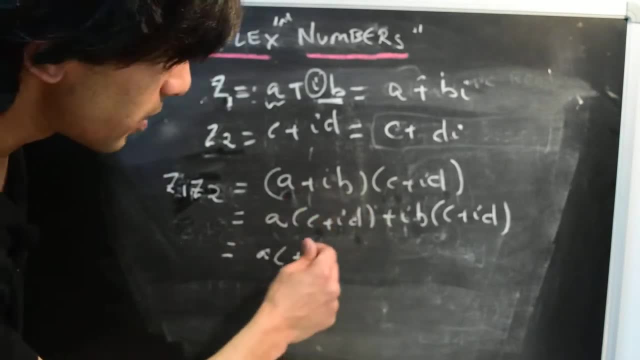 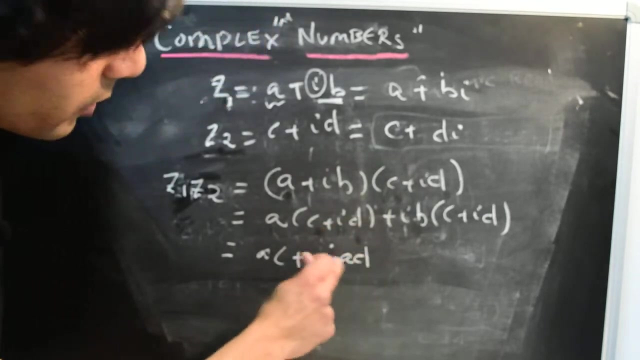 what we'll say is: we can distribute this multiplication over addition. So this gives us A times C, plus again we'll sort of we'll allow I to commute with the real numbers that it's operating with. so we have I times AD. So we could have written I anywhere in this expression. so just 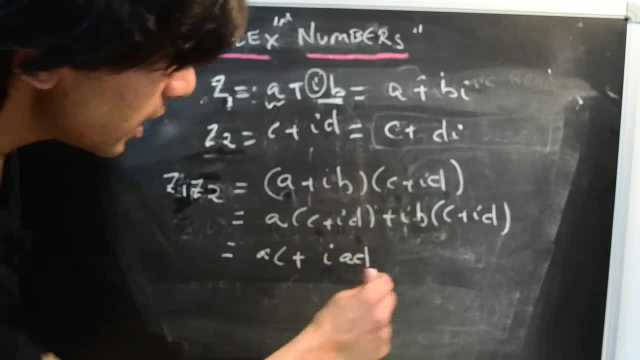 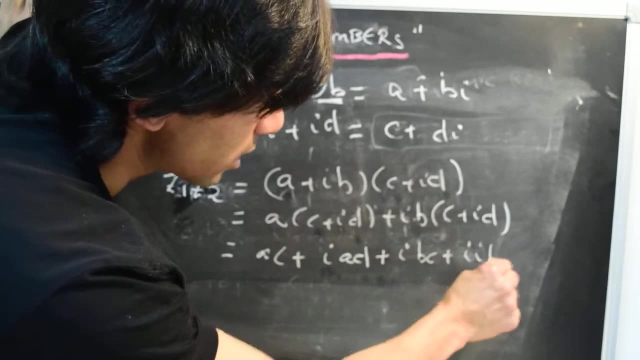 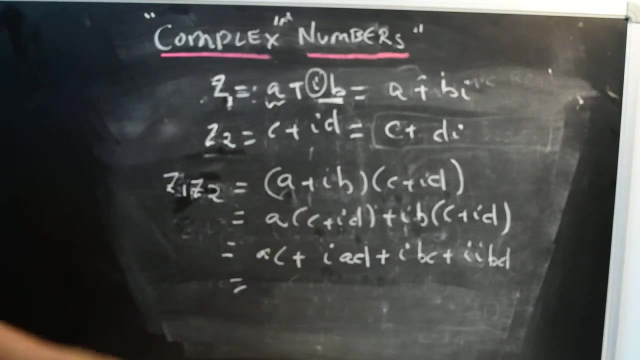 for simplicity, I'm writing it as the first symbol, so I times AD, and then we have I times BC, plus I times I times B times D. Okay, so again we'll do the same thing as we did in when we when we were adding complex numbers, is to identify in this expression the real 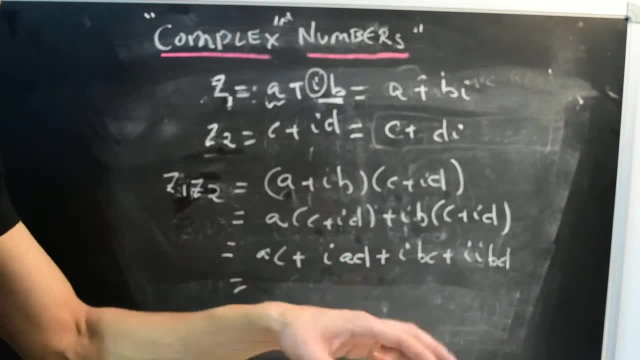 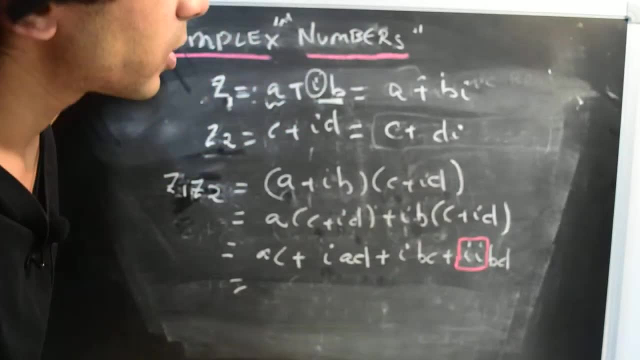 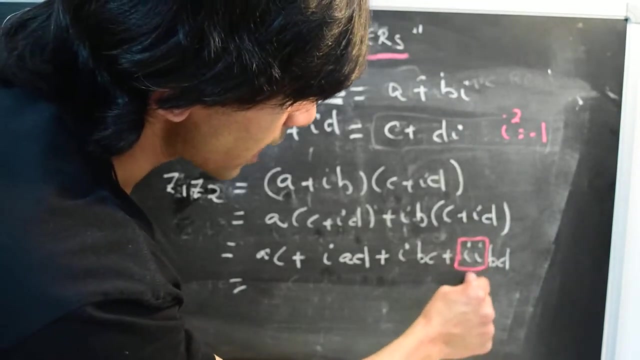 numbers and the expression that appeared with the symbol. I Now notice that here we have an I square or an I times I, and we know that I square is minus of 1 and minus 1 is a real number. so this I times I is actually minus of 1 and therefore we can combine it with. 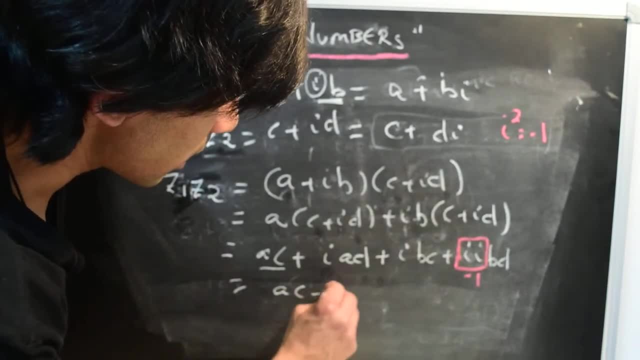 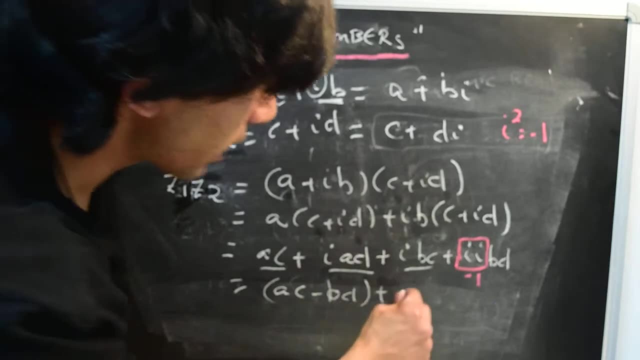 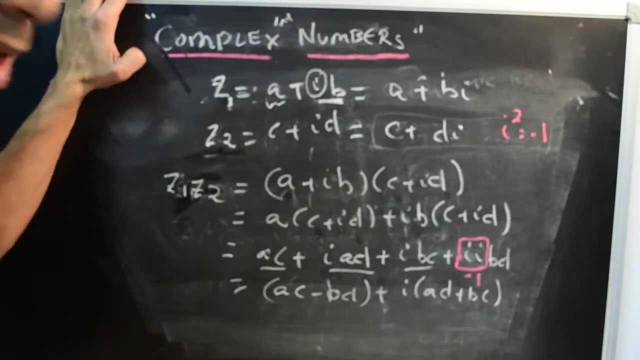 A times C, to write this as A times C minus I times B plus I times B plus I times B plus I minus B times D plus. Now these two carry a single unit, I, and so we can write this as I times AD plus BC. Okay, so with this definition of multiplication, what we find is that the 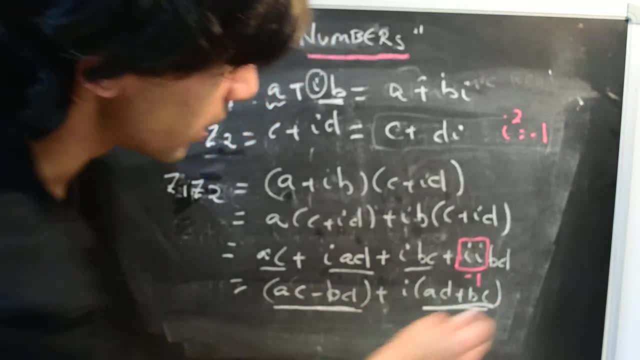 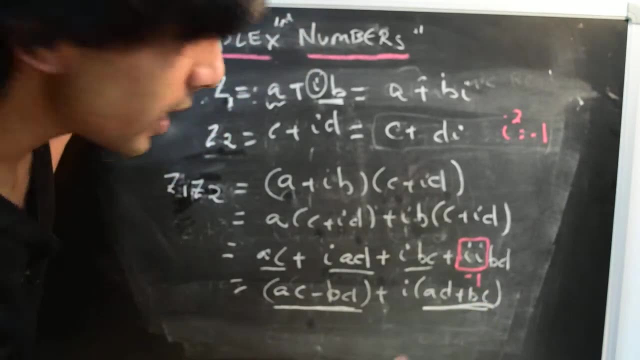 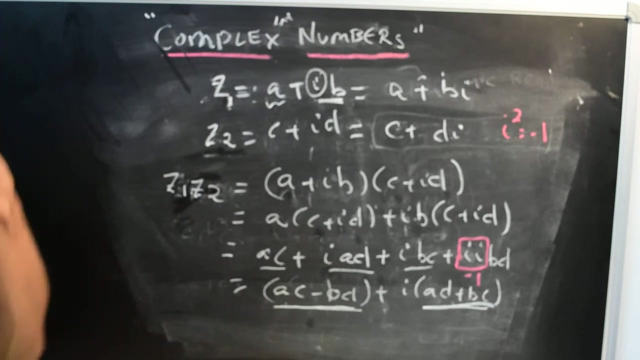 end result is another sort of object that looks like a complex number, because we have a real part which is AC minus BD plus I times an imaginary part, AD plus BC, And these two parts are both real. So this sort of object is another complex number And likewise we can check that this. 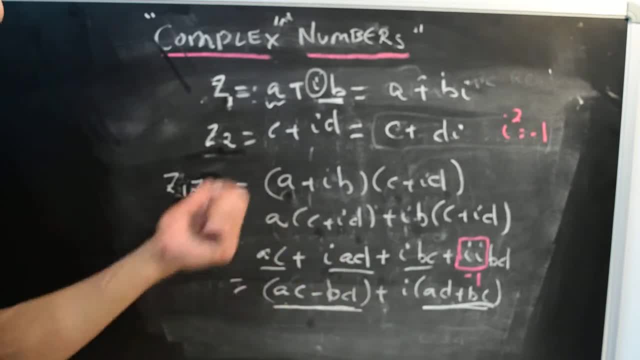 Z1- Z2. with this definition of multiplication, Z1- Z2 is actually equal to Z2 times C1.. So it turns out that if we make this definition, then complex the multiplication, this definition for multiplication of complex numbers, then multiplication of complex numbers also commutes. 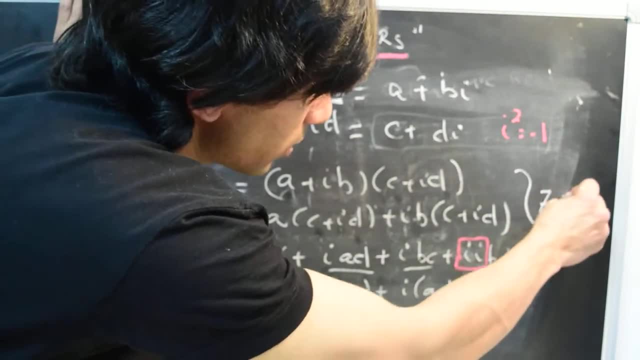 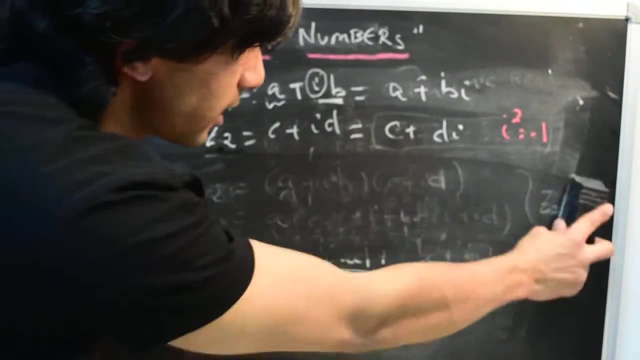 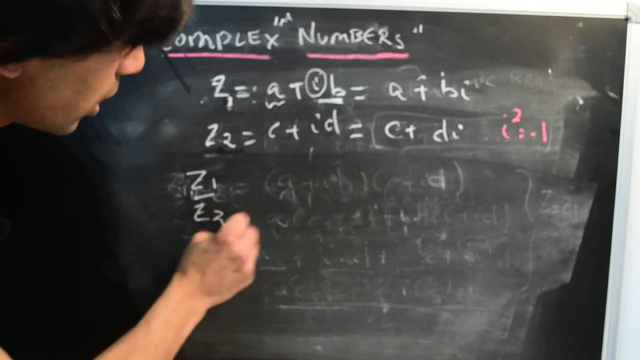 So that's something that one should check. So this it will turn out to be equal to Z2 times C1.. Okay, And the last step is to define division of complex numbers. So Z1, let's say, divided by Z2, provided Z2 is non-zero. So what does it mean for a complex number to be non-zero? 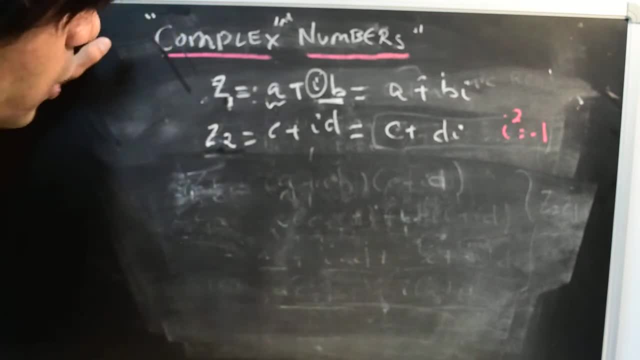 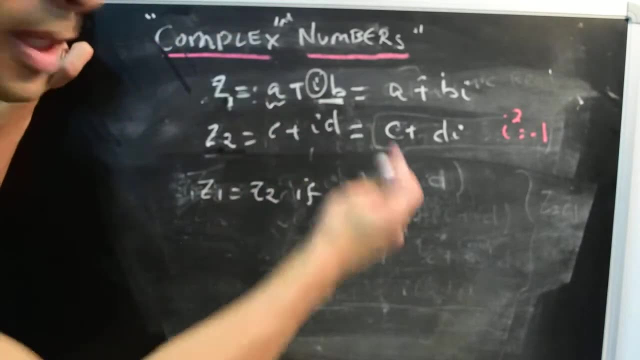 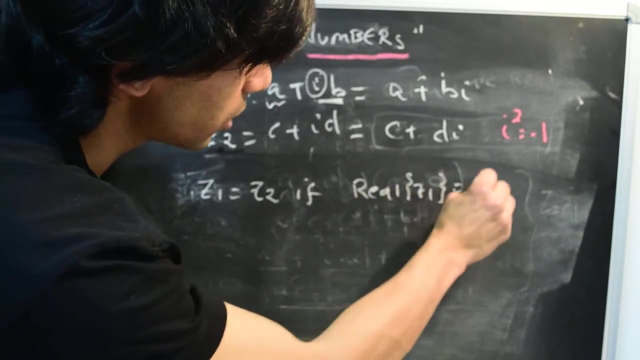 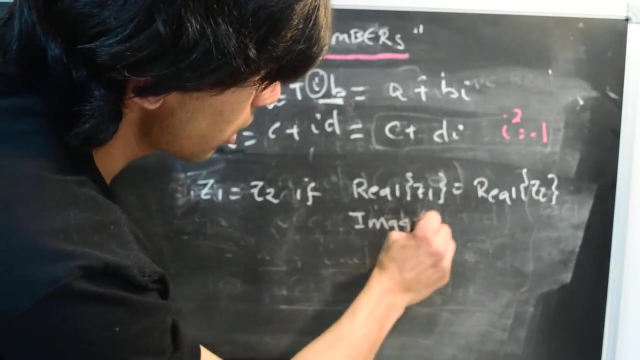 A complex number is actually. let's do that first. Two complex numbers are equal to each other, So Z1 is equal to Z2.. If their real paths are equal and their imaginary paths are equal, So if real part of Z1 is equal to real part of Z2 and the imaginary part of Z1 is. 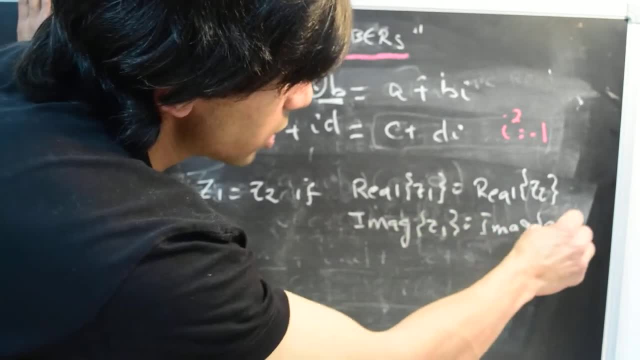 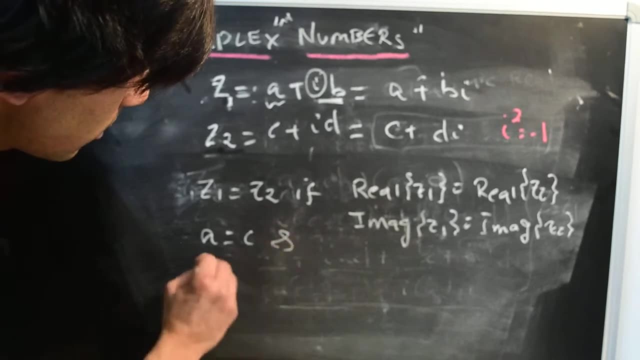 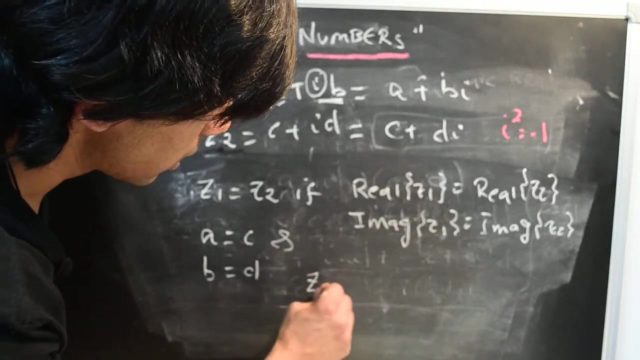 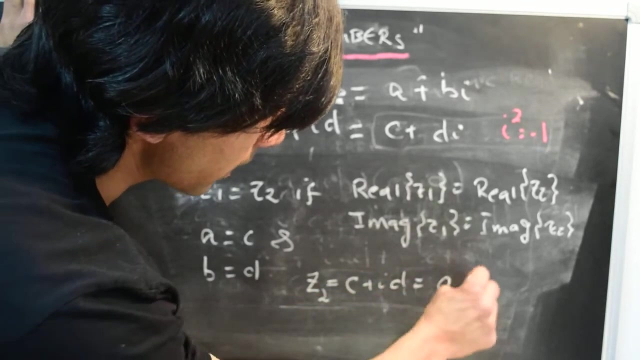 equal to the imaginary part of Z2.. So in this case, these two complex numbers are equal. if A equals C and B equals D, So a complex number is zero. Let's say Z. in this case, let's pick out Z2.. So Z2 is zero. if so, zero has only a real part, which is zero. If C is zero and 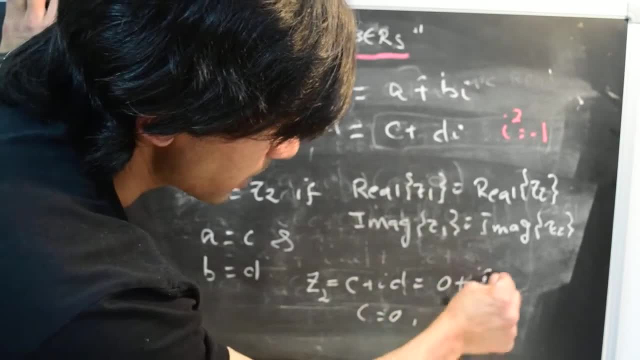 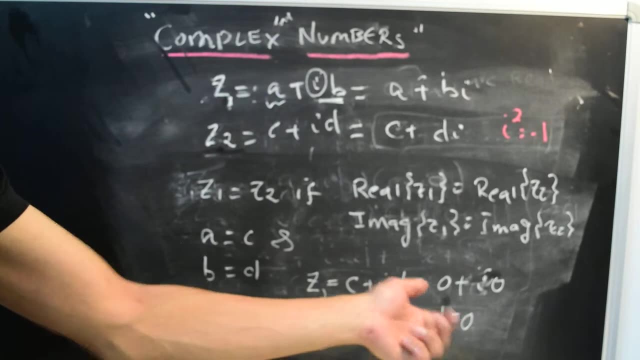 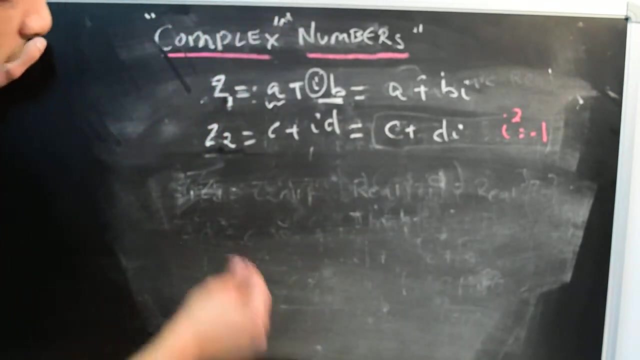 or we can input. in fact we can write this as zero times I times zero. So if C is zero and D is zero, So a complex number is zero if both its real part is identically zero and its imaginary part is identically equal to zero. So if Z2 is non-zero, we can divide Z1 by Z2 and write: 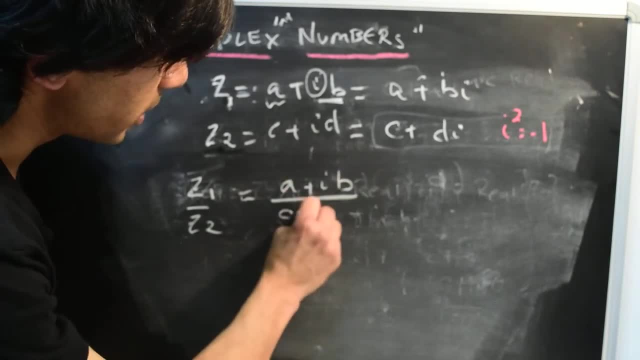 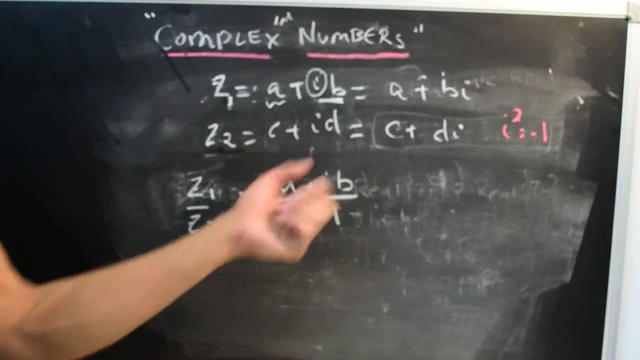 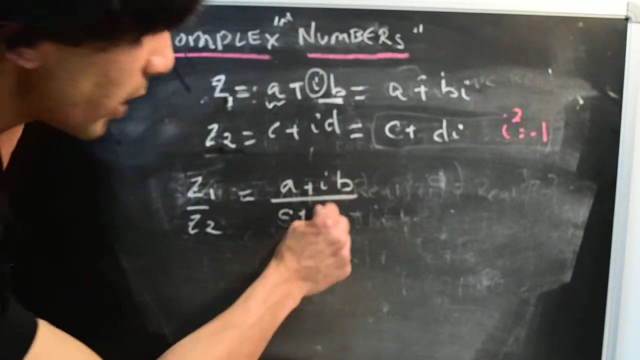 it as A plus IB, divided by C plus ID. Now again what our aim is: to write this sort of expression in the form of a real part plus I times an imaginary part. So we need somehow to get rid of the I in the denominator here, and one way to do that is to multiply the. 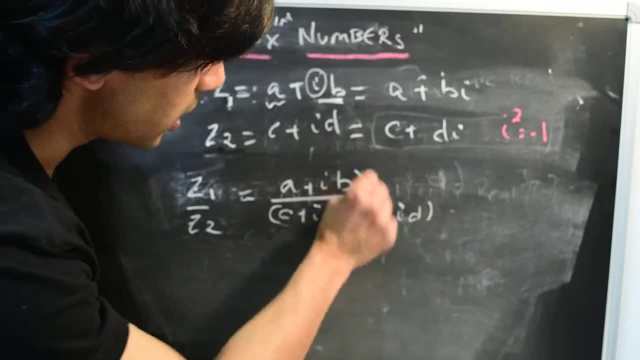 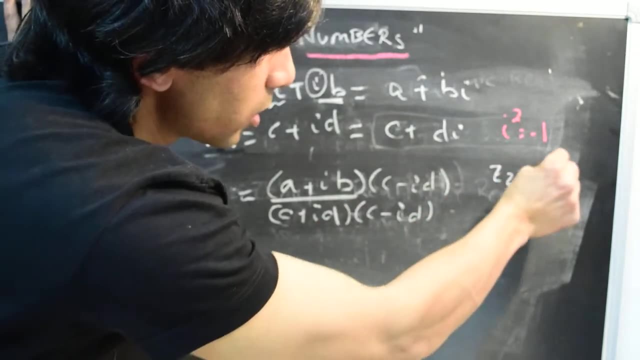 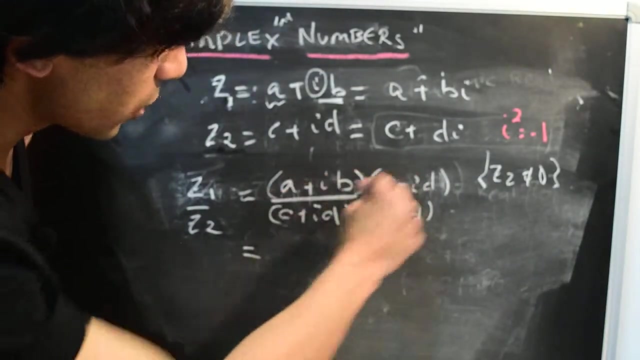 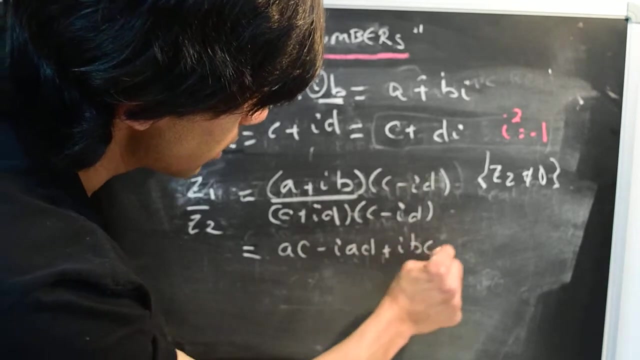 numerator and denominator with C minus I times D. And again we are saying that Z2 is non-zero, so that's important. So again we can carry out the product in the numerator and the denominator. So in the numerator we'll find that this is AC minus I times AD plus I times BC minus. 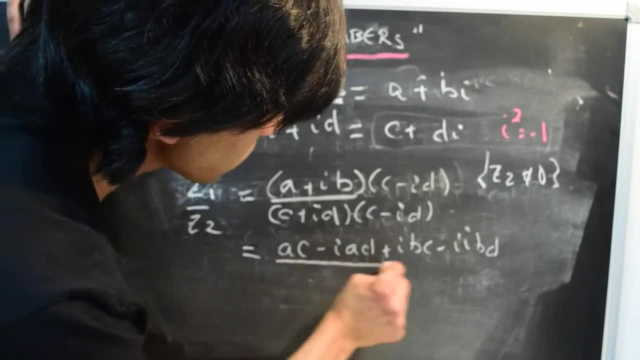 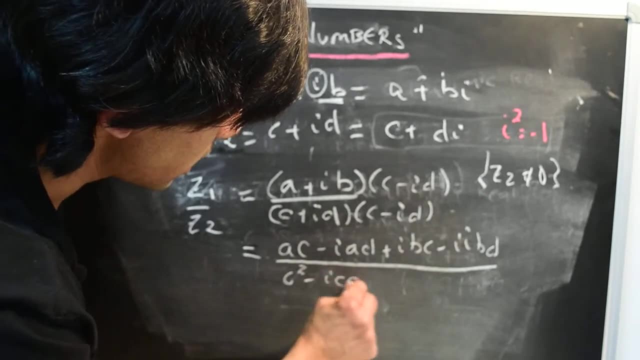 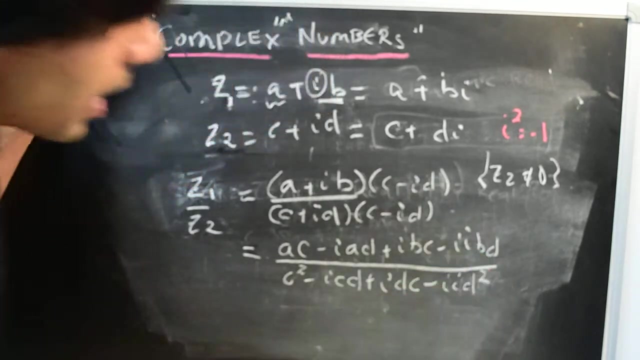 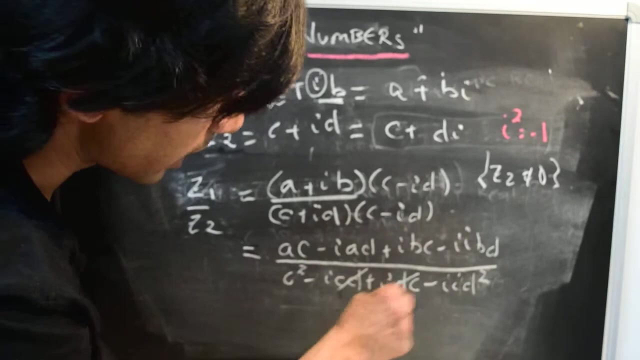 times i times bd, and in the denominator we have c times c, which is c square minus i times c times d plus i times d times c minus i times i times d square. Now again the real numbers sort of commute. so this minus i times cd is actually equal to i times dc, so this cancels. 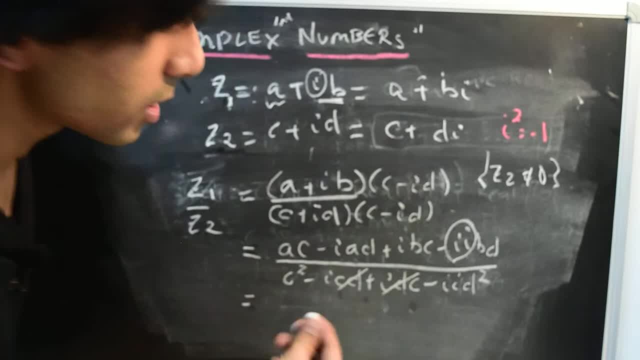 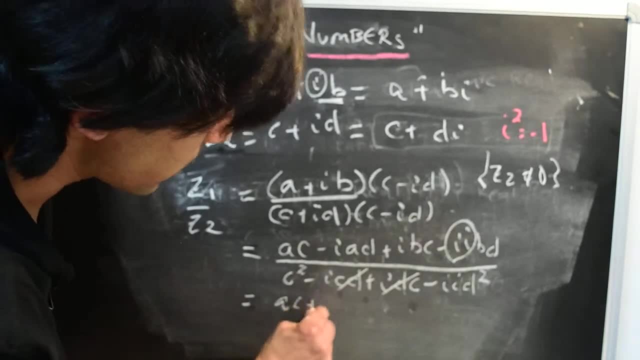 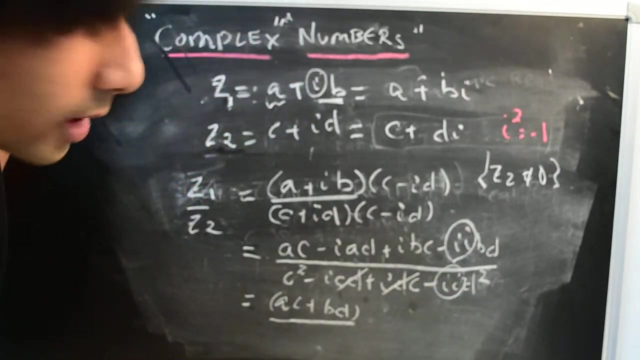 out and in the numerator we have an i square here which is minus a one. so overall we have a plus sign here, because this minus minus gives us a plus. so we have ac plus bd and the denominator. we also have an i square which will give us a minus one, and then we have